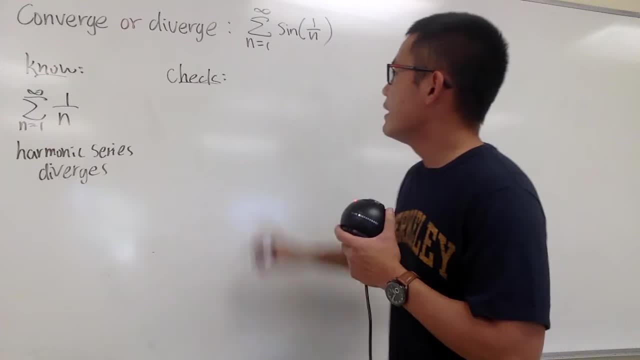 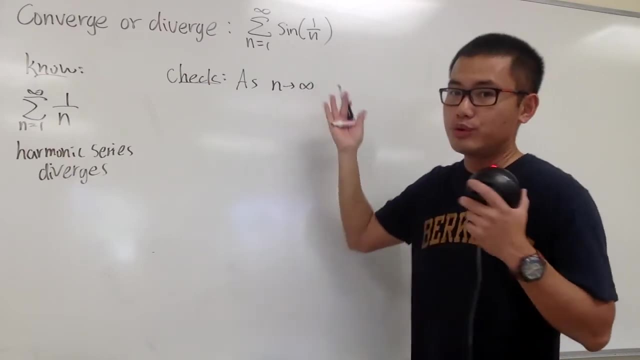 So here is the check And, as usual, we are going to check the limit, as n goes to infinity. And let me just write this down for you guys: If I put down n goes to infinity, that's how we usually would do it, alright. 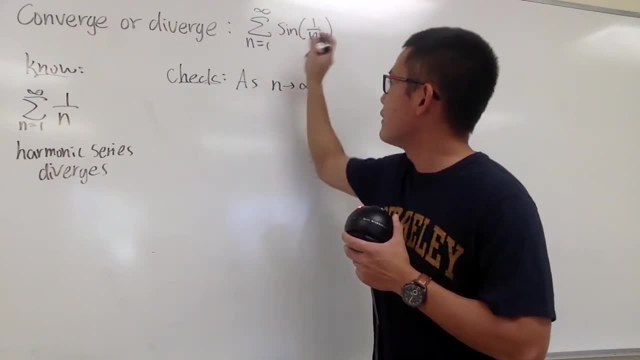 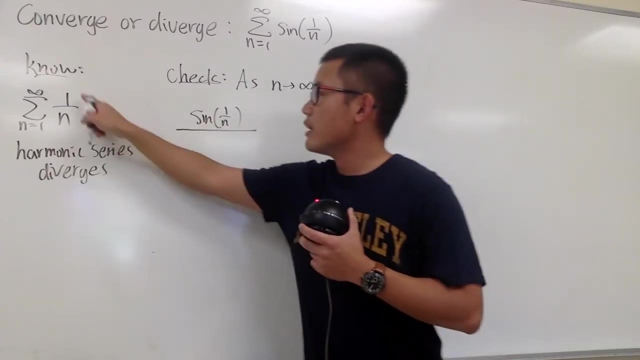 And I'm just going to put down the original right here on the top, which will have sine of 1 over n, And then we will divide this by this- The things that we know much better- which is 1 over n, right. 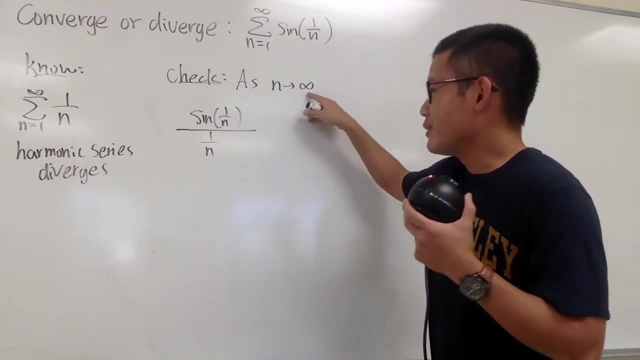 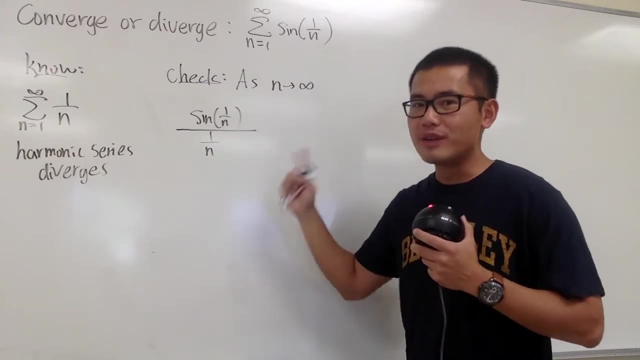 Okay, how can we check the limit of this? Technically, we can still plug in infinity into the n here. right On the top, you get 0.. On the bottom, you also get 0. This is a 0 over 0 situation. 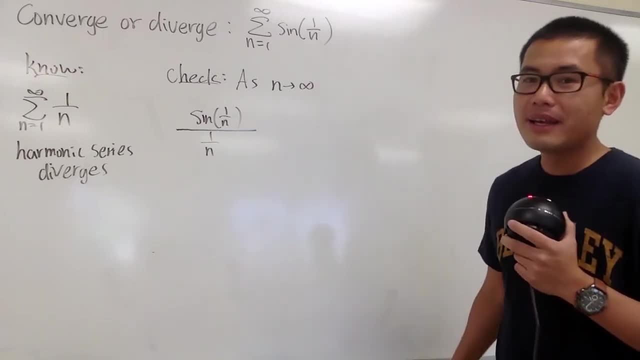 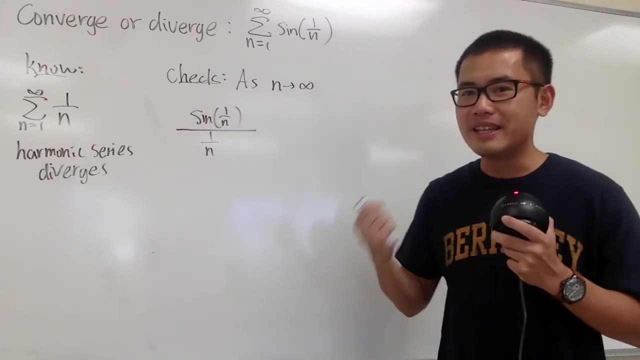 So what do we do? Well, to utilize L'Hopital's rule, right. But the problem with this is that we cannot put down d, dn, We cannot differentiate with respect to n, because n is technically just a bunch of whole numbers. 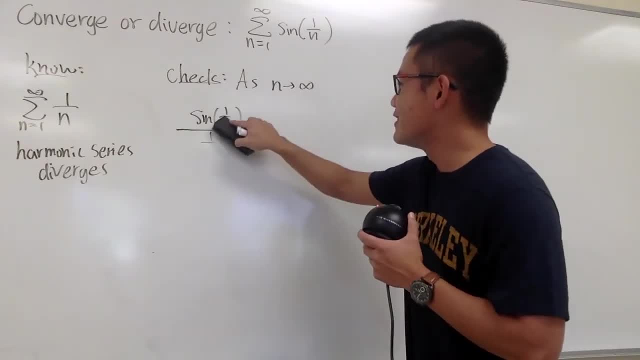 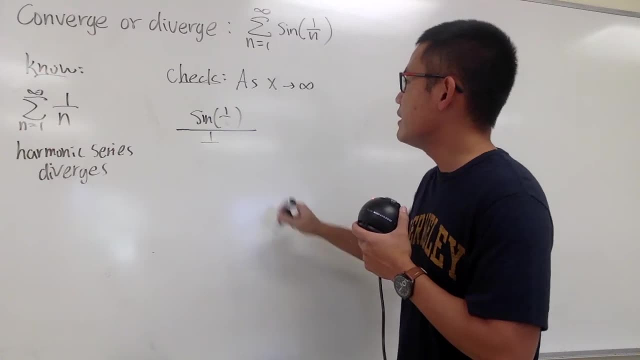 So, with that being said, in our case here, I'm going to actually change this to x, So I can legitimately use the L'Hopital's rule. So x goes to infinity. Let's check sine of 1 over x over 1 over x. 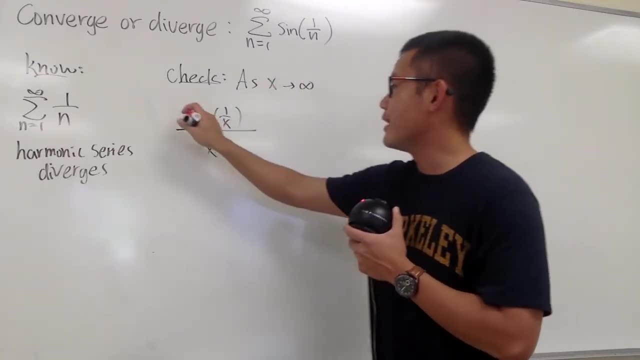 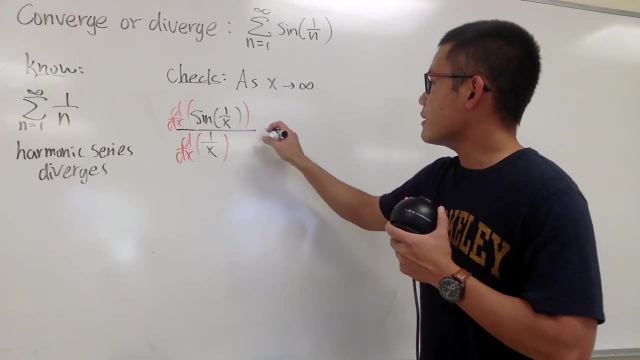 And we still have 0 over 0.. But we can use L'Hopital's rule now And we can just put down d, dx, d dx. alright, Okay, So I will draw. I'm going to draw an arrow. 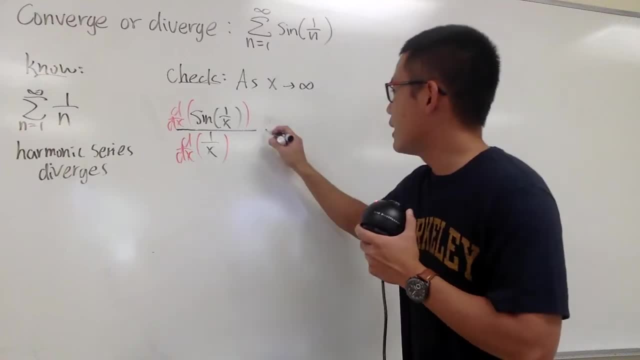 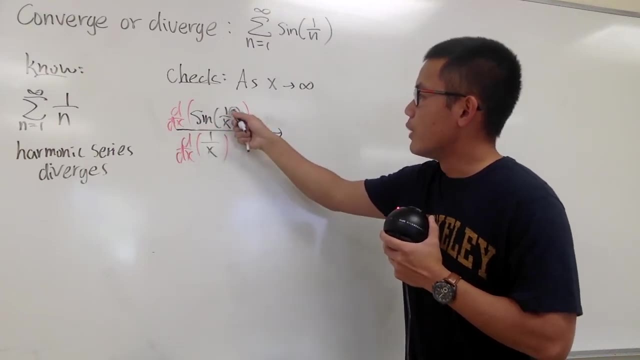 Well, actually I'm just differentiating. Well, I'm going to draw an arrow because this is going to be approaching to what happens next, right Anyway, here, when we do the sine of 1 over x- derivative sine, we know it's cosine. 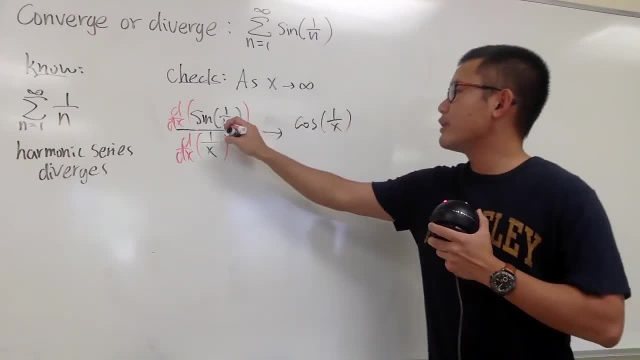 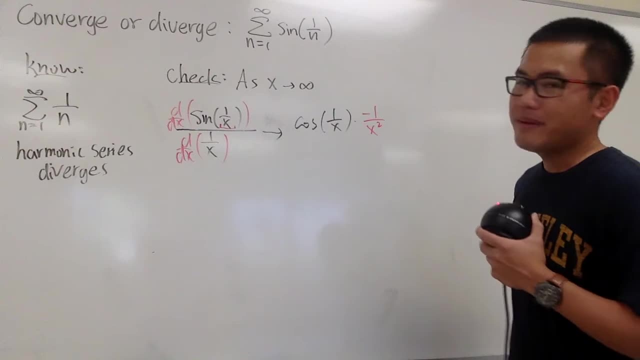 And the input state is the same, which is 1 over x, But we have to multiply by the derivative inside. The derivative of 1 over x is negative. 1 over x squared okay, And this is over. We differentiate 1 over x. 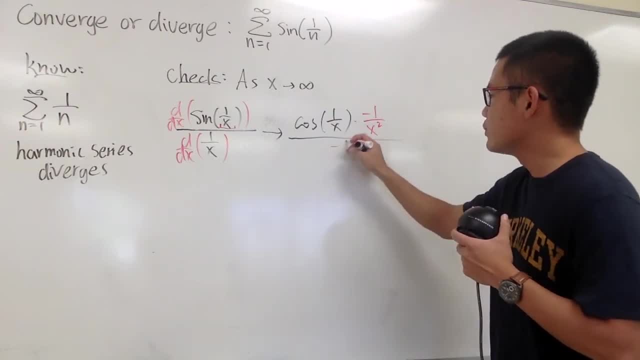 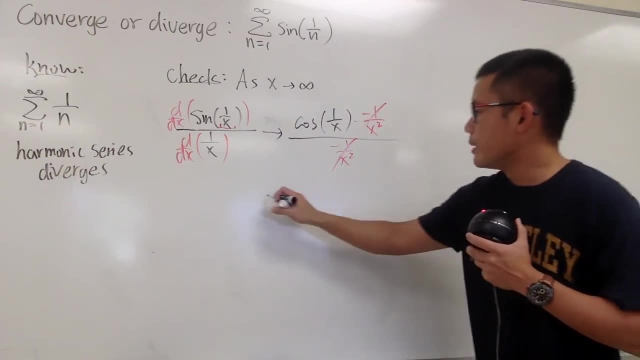 And it's just the same as that, right. So the derivative of 1 over x is negative, 1 over x squared. And you see this and that cancel each other out completely. And you see this is going to be approaching to cosine of 1 over x.